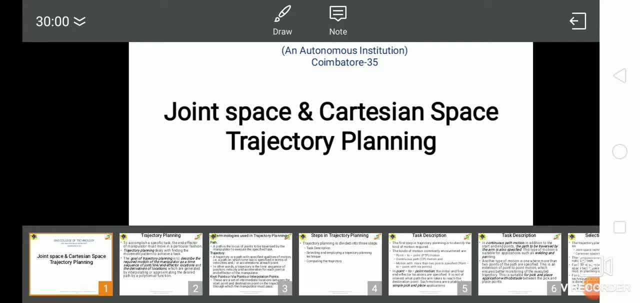 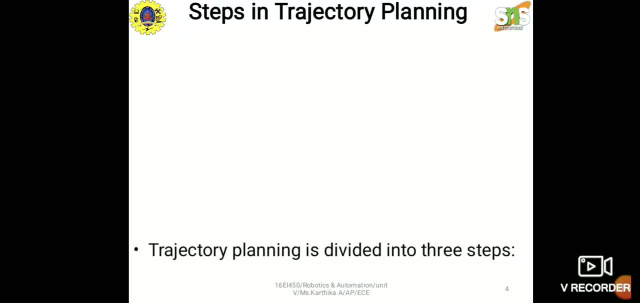 Next steps in trajectory planning. First one is task description. Next one: selecting and employing a trajectory planning technique. Third one is computing the trajectory. Next one is task description. Next one is selecting and employing a trajectory planning technique. Next one is task description. Next one is task description. What is task description? 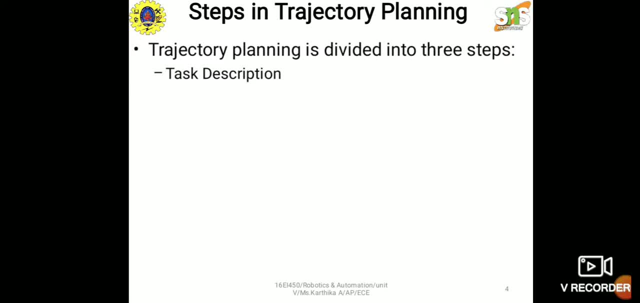 The first step in trajectory planning is to identify the kind of motion required. The kinds of motion commonly encountered are point-to-point motion, continuous path motion and motion with more than two points specified. point-to-point with via points. First, what is point-to-point? 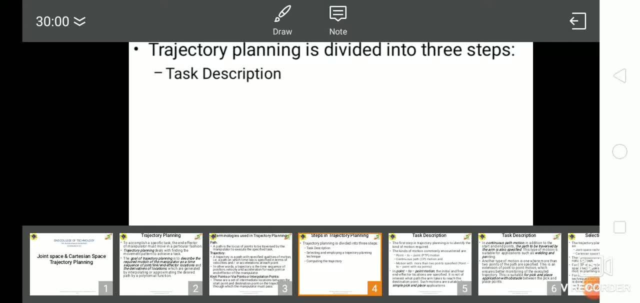 motion, The initial and final end effector locations are specified. It is not always known what the path arm takes to reach the destination point. Such motions are suitable for simple pick-and-place applications. Next one: in continuous path motion, in addition to the start and end points, the path to be traversed by the arm is also specified. This 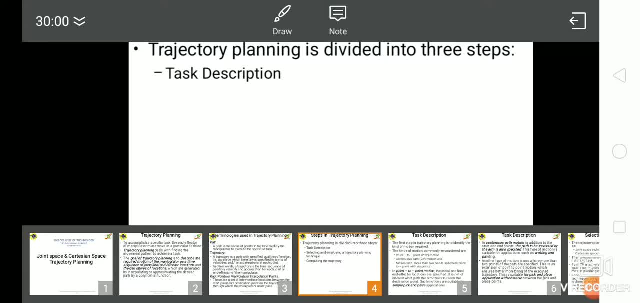 type of motion is suitable for applications such as welding and painting, And the type of motion is one where more than two points of path are specified. This is an extension of point-to-point motion which ensures better monitoring of the executed trajectory. This is suitable for pick-and-place application with obstacle between pick and place points. 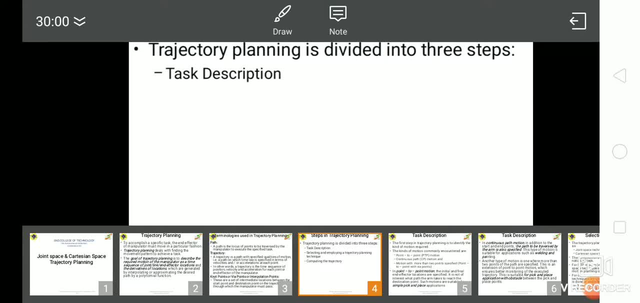 First, selection techniques in trajectory planning. In this we have two types. First one is joint space techniques, second one is Cartesian space techniques. The selection of the technique depends on the nature of the task. For P2P motion with or without via. 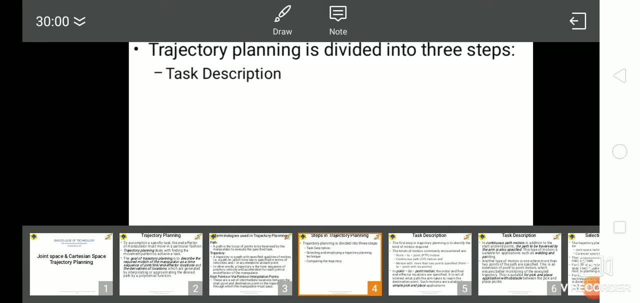 points techniques are employed wherein the motion plan is done at joint level. For contrives path motion, Cartesian space techniques are used wherein the motion planning is done at end-effector level. In this case, the joint variables required to achieve a desired end-effector location is calculated from inverse kinematics. 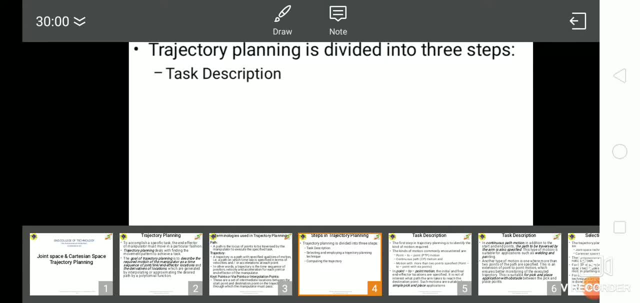 Next, how to computing the trajectory. The final step in trajectory planning is to compute the time sequence of values attain by the function generated from the trajectory planning technique. We already know we have two types. First, one is joint space. Second, one is cartesian spaceWhat's the 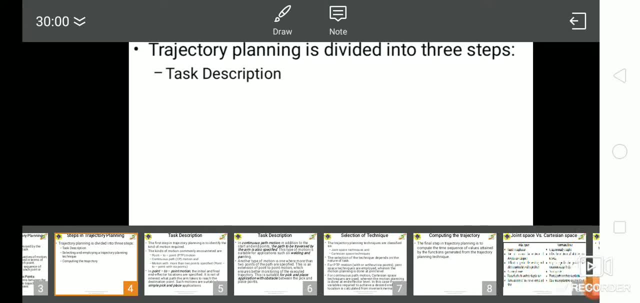 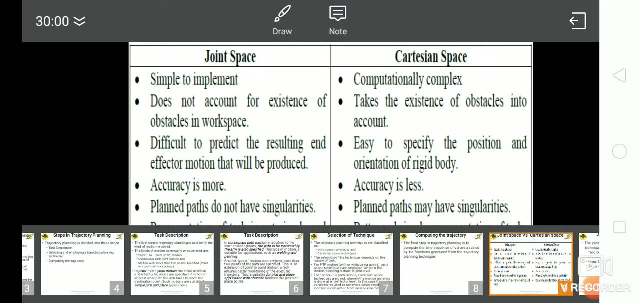 difference between joint space and cartesian space. First, joint space: it is simple to implement. cartesian space: It is computationally complex. Joint space does not account for existence of obstacles in workspace space. In Cartesian space, it takes the existence of obstacles into account. 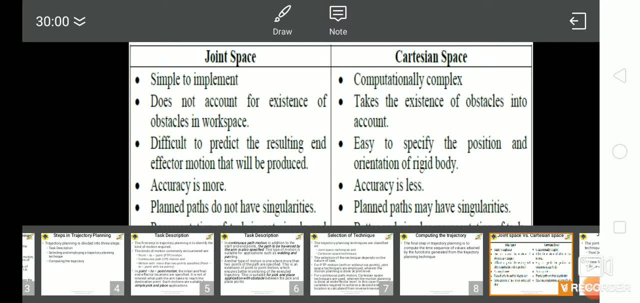 Joint space is difficult to predict the resulting end-effector motion that will be produced. In Cartesian it is easy to specify the position and orientation of rigid body. Here in joint space the accuracy is more. In Cartesian the accuracy is less. 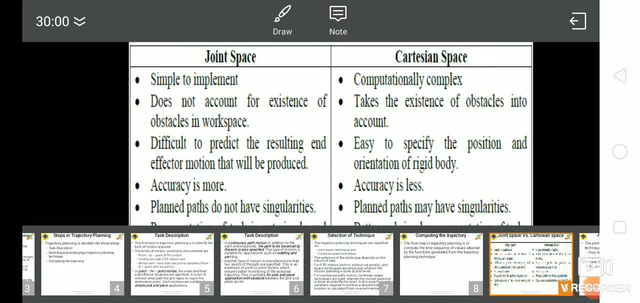 In joint space. the planned paths do not have singularities In Cartesian space. the planned paths may have singularities In joint space. the representation of task is not simple and clear In Cartesian. it is better and simpler representation of task. 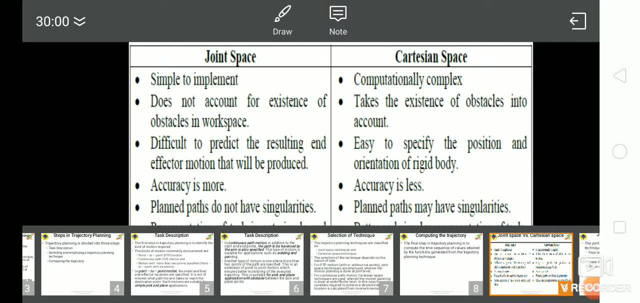 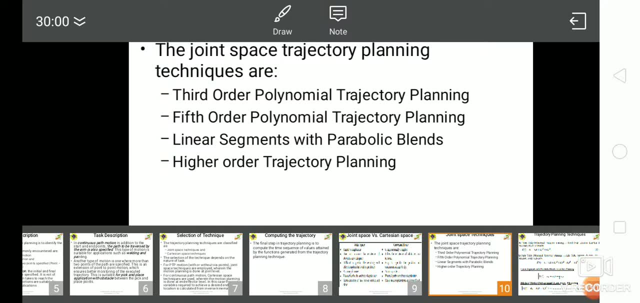 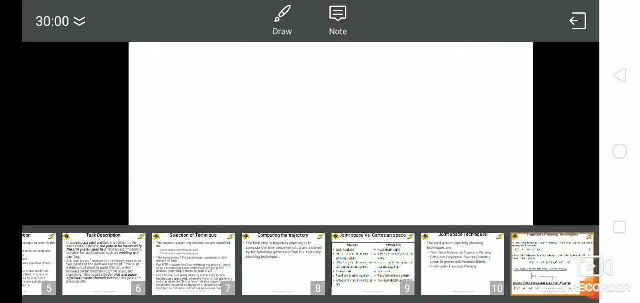 Next, joint space techniques. The joint space trajectory planning techniques are: third-order polynomial trajectory planning. fifth-order polynomial trajectory planning, linear segments with parabolic blends. higher-order trajectory planning. In third-order polynomial trajectory planning, a third-order equation describes the trajectory which is given by: 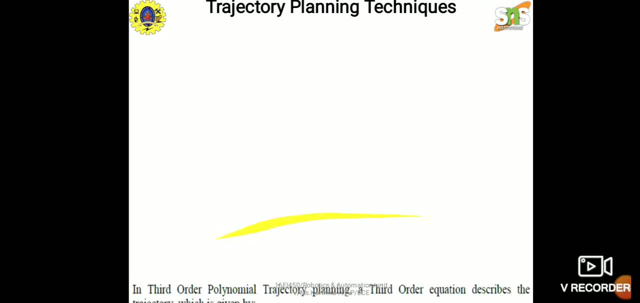 theta of t equal to a naught plus a 1 t plus a 2 t squared plus a 3 t cube In fifth-order polynomial trajectory planning. a fifth-order equation describes the trajectory which is given by theta of t equal to a naught plus. 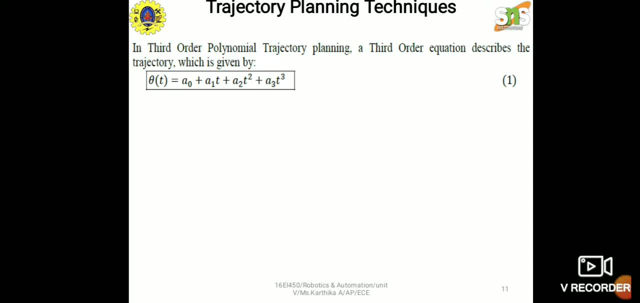 a 1 t plus a 2 t squared plus a 3 t cube plus a 4 t power 4 plus a 5 t power 5.. Third-order uses third-order polynomial trajectory planning. For fifth-order we can use fifth-order trajectory planning. 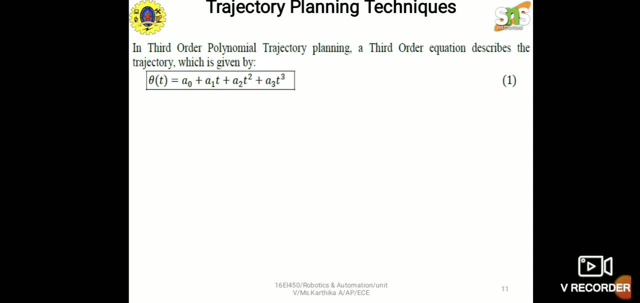 Linear segments with parabolic blends. trajectory planning contains theta of t equal to a naught plus a 1 t plus 1 by 2 a 2 t squared In higher-order polynomial trajectory planning: theta of t equal to a naught plus a 1 t plus a 2 t squared plus etc. plus a n minus 1 t power. n minus 1 plus a n t power. 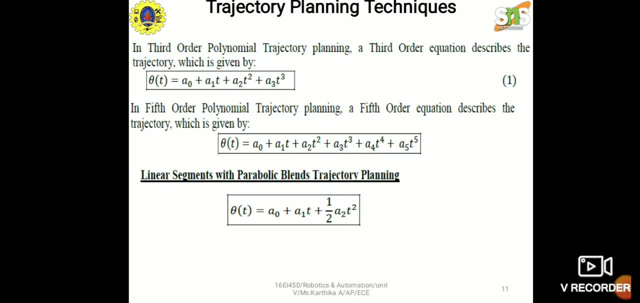 n for n-th-order polynomial trajectory planning. Next: joint space techniques- Linear segments with parabolic blends. trajectory planning contains theta of t equal to a naught plus a 1 t plus 1 by 2 a 2 t squared In higher-order polynomial trajectory planning: theta of t equal to a naught plus a 1 t plus a 2 t squared plus a n minus 1 t. power n minus 1 plus a n t. power n for n-th-order polynomial trajectory planning. 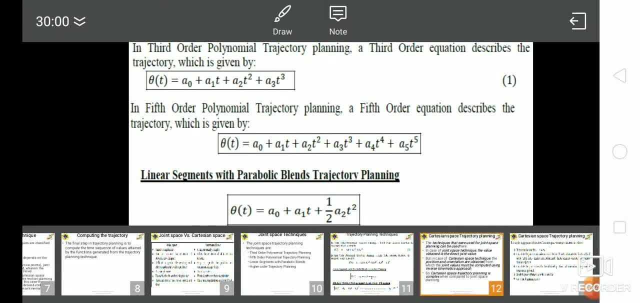 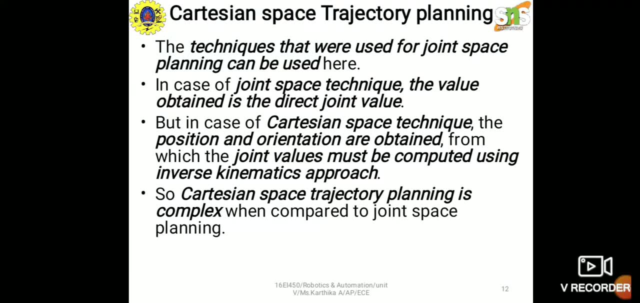 Next, Cartesian space trajectory planning. The techniques that were used for joint space planning can be used here. In case of joint space technique, the value obtained is the direct joint value, But in case of Cartesian space technique, the position and orientation are obtained, from which the joint values must be computed using inverse kinematics approach. The techniques that were used for joint space planning can be used here. In case of joint space technique, the value obtained is the direct joint value, But in case of Cartesian space technique, the position and orientation are obtained from which the joint values must be computed using inverse kinematics approach. 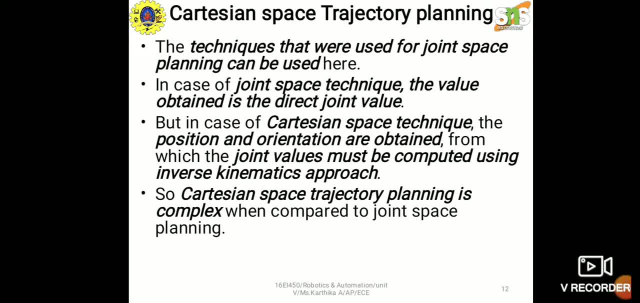 The techniques that were used for joint space technique: the value obtained is the direct joint value, But in case of Cartesian space technique, the position and orientation are obtained from which the joint values must be computed using inverse kinematics approach. The techniques that were used for joint space technique: the value obtained is the direct joint value, But in case of Cartesian space technique, the position and orientation are obtained from which the joint values must be computed using inverse kinematics approach. 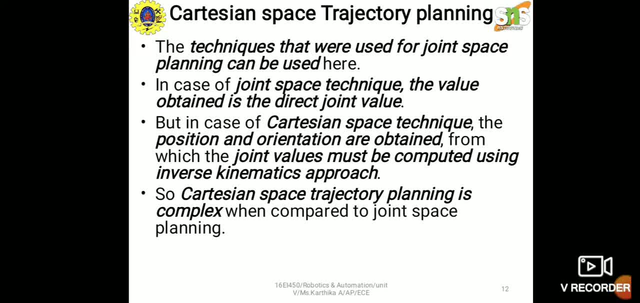 So Cartesian space trajectory planning is complex when compared to joint space. The step by step process followed in Cartesian space planning is described as follows. The first step is Incremented time by t equal to t plus delta t. The second step is Incremented time by t equal to t plus delta t. 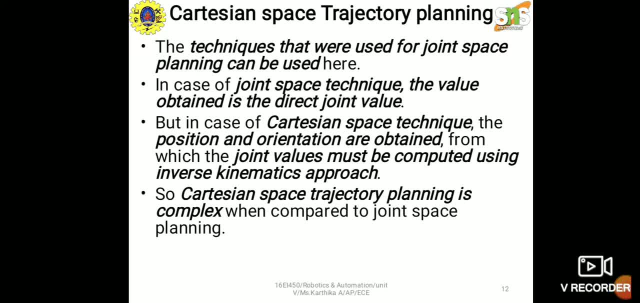 here, delta is variation in time. second step: step to us to calculate the position orientation of the hand based on the selected function: third order or fifth order or higher order, polynomial or linear segment, with parabolic blends for the trajectory. next, to calculate the joint values for the obtained position and orientation using inverse kinematics approach. next, send the joint. 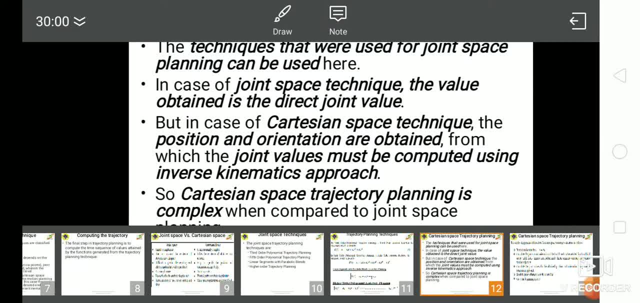 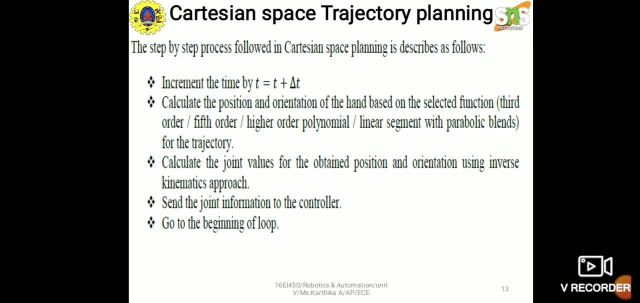 information to the controller. the last one is go to the beginning loop. okay, i repeat again. first, increment the time by t, equal to t plus delta t. second one is: calculate the position and orientation of the hand based on the selected function. it may be. third order, fifth order.